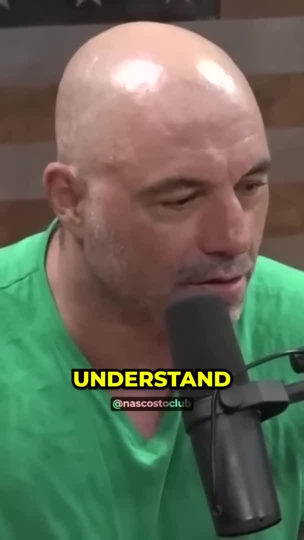 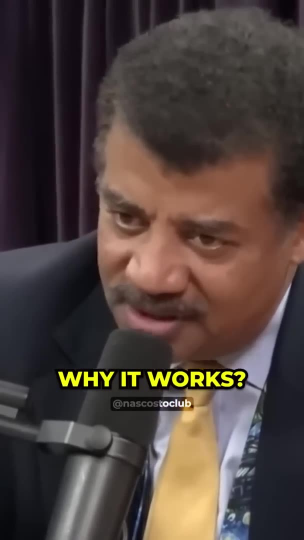 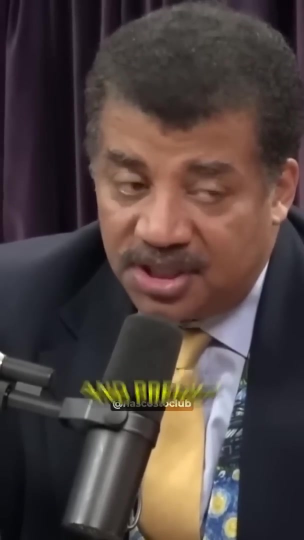 Gravity. One of the things that confuses me the most is that we don't really understand what gravity is. Science can describe how gravity works, but can they describe why it works, Can we? So this is the how-why duality here In science: if we can describe how something works and predict its future. 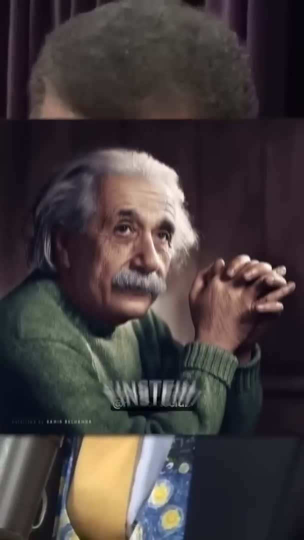 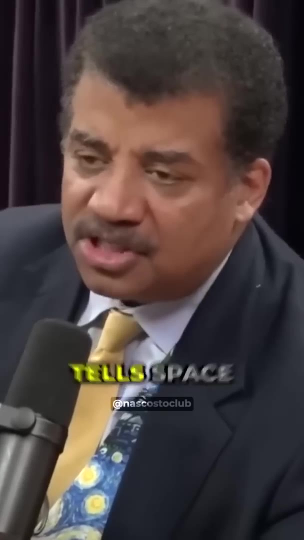 behavior. we claim to understand it and we move on. Get to Albert Einstein. Gravity is the curvature of space and time and you're moving on the curvature of that fabric. That's gravity. Matter tells space how to curve. Space tells matter how to move. I can describe what gravity is doing. I. 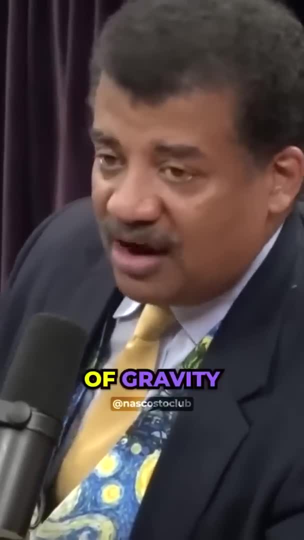 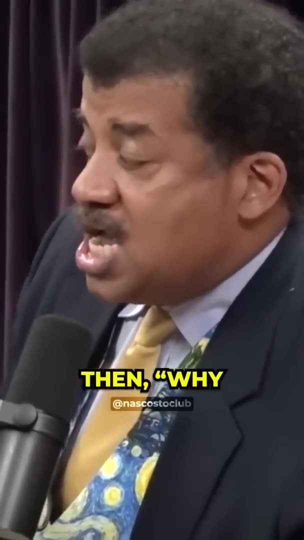 even have a mechanism for it. You say: why did it fall? I say there's a force of gravity operating on it. Why did it fall that way? Because of the curvature of space and time. I'm answering your whys. I understand Then. well, why does matter and energy curve space and time? Okay, that's a. frontier. We're still working on that. 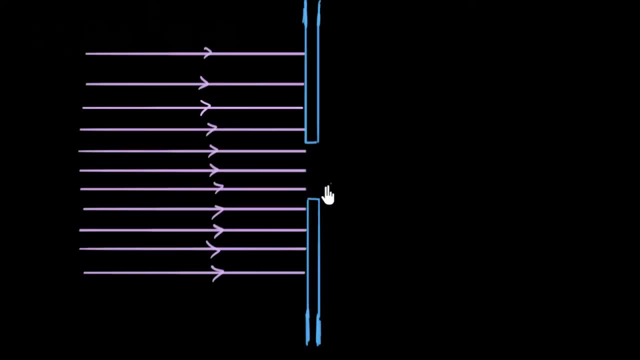 If you shine a parallel rays of light on a cardboard with a tiny hole in between, what would you expect to happen to this light after it went through the hole? Well, if you think in terms of Newton's idea where light is a bullet, then we'll all see. 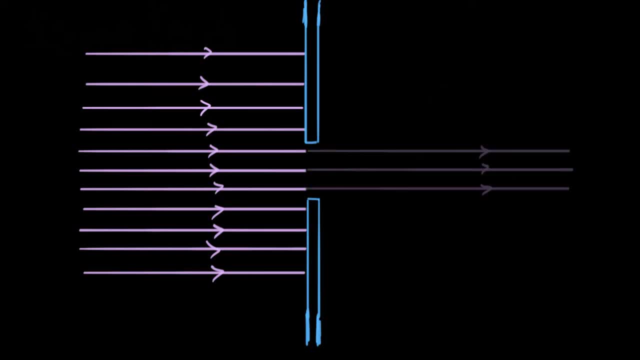 that these bullets will get blocked and these bullets will just go straight through And this is the picture that gets painted. But careful experiments show that when the light goes through the hole, it actually spreads out and forms a bigger spot. if there was a screen over here. 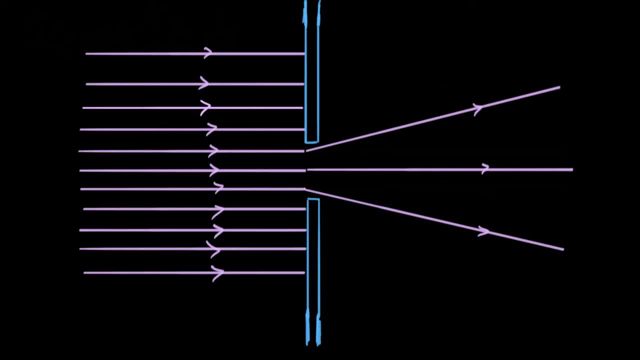 How do you explain that? How does light just bend like that? Well, if you think of light as a wave and use Huygens' principle, then we'll be able to explain this, And that's pretty much what we want to do in this video.